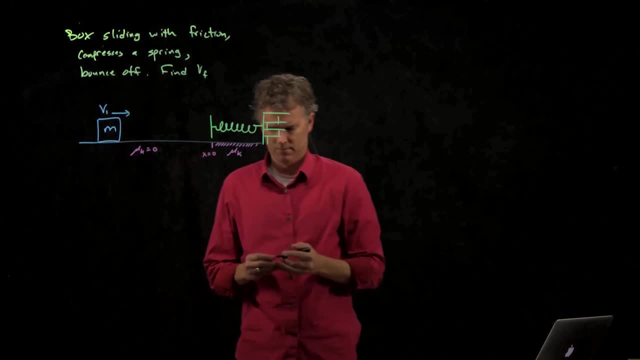 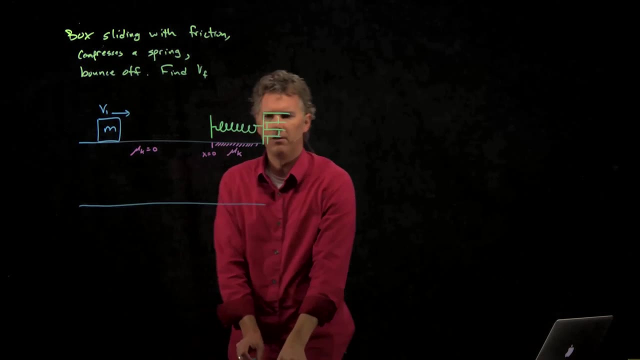 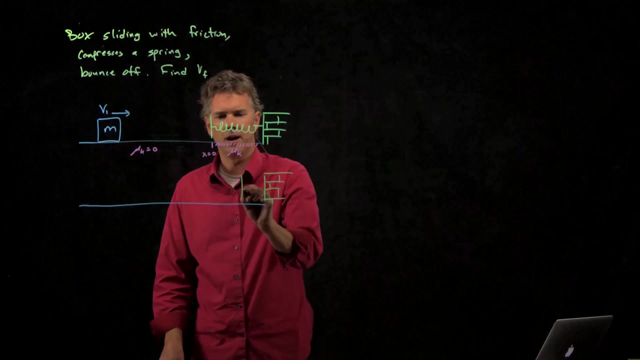 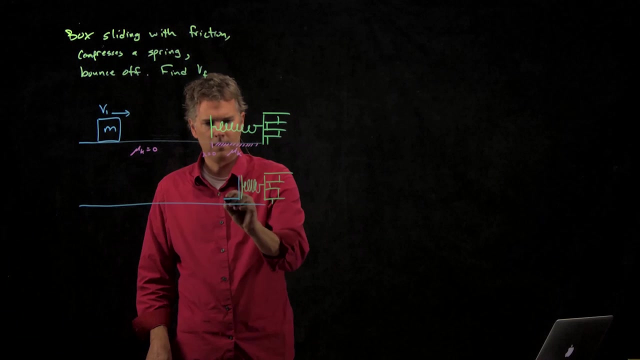 And we can call this position x equal 0.. So let's draw the second picture, where it has compressed the spring. So here is our brick wall. The spring is now compressed, It's all coiled up. Box is right against it. 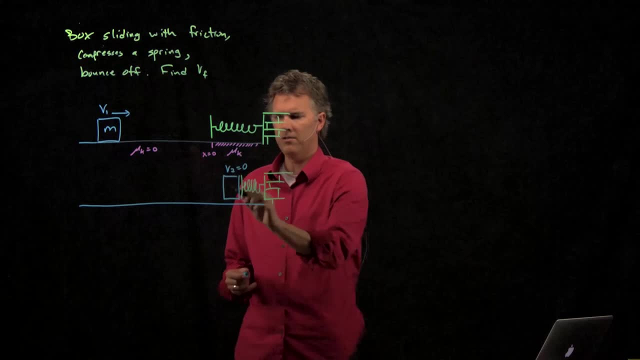 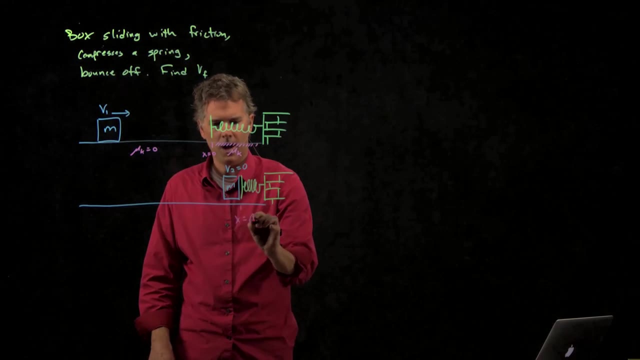 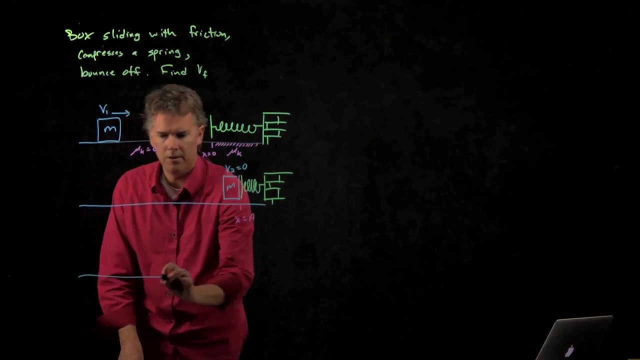 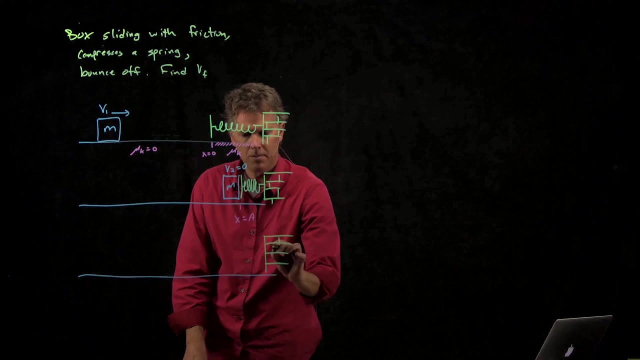 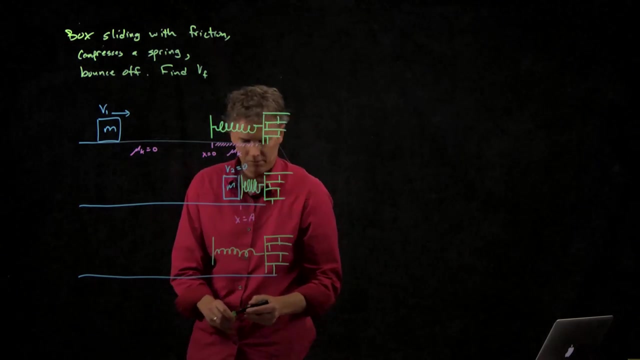 V2 is 0.. It's come to rest momentarily And this is at a position x equals a, And now, in the third part of this, the box bounces back off and shoots back out. So spring comes back out to its full length. back to x equals 0.. 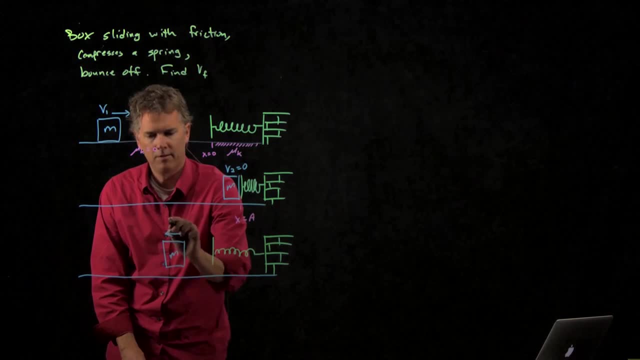 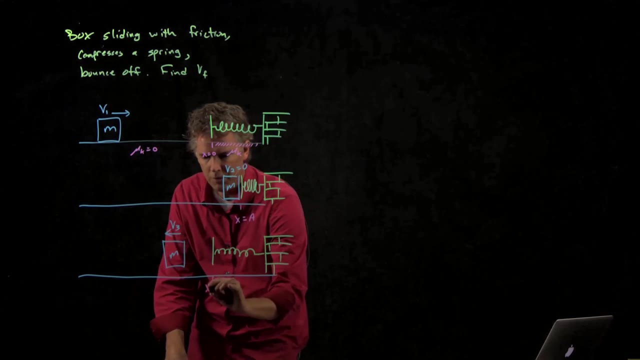 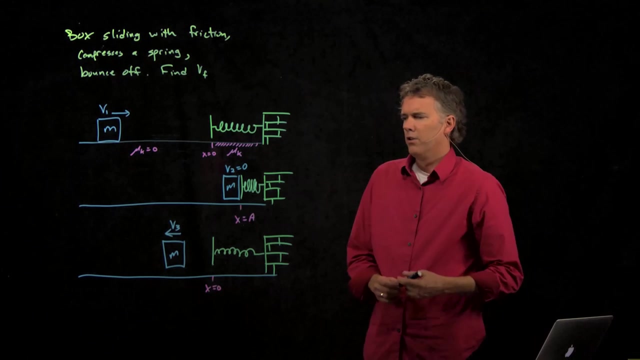 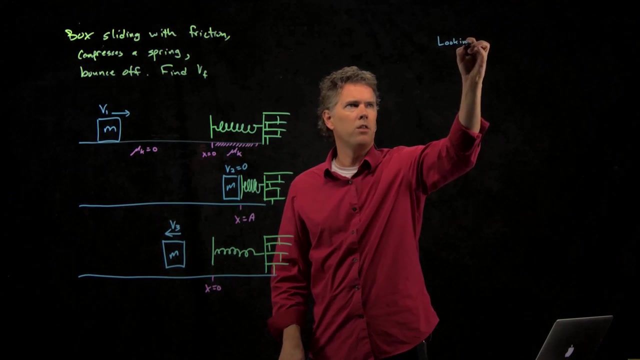 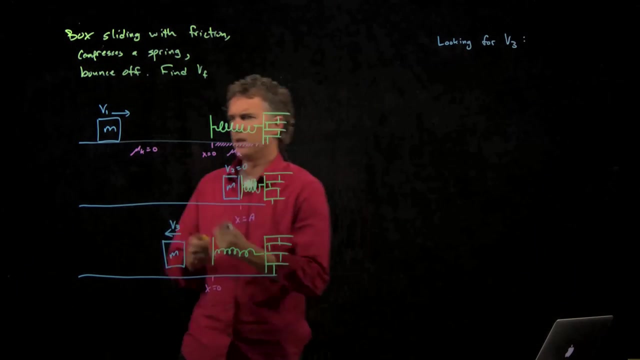 Box M takes off at V3. And the spring, of course, returns to its normal equilibrium position. So let's find V final, which means we are looking for V3. And so this is going to be position 1.. This is position 2.. 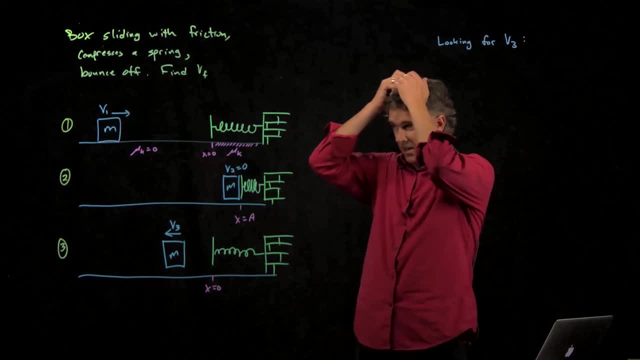 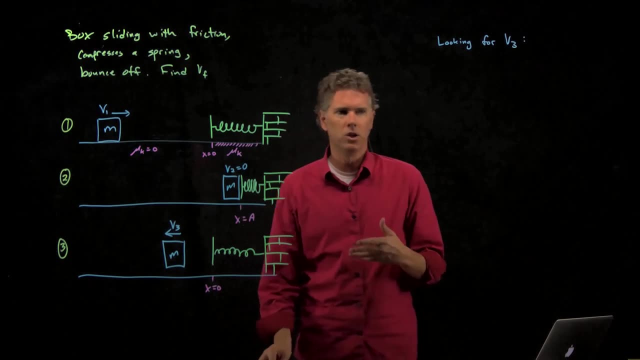 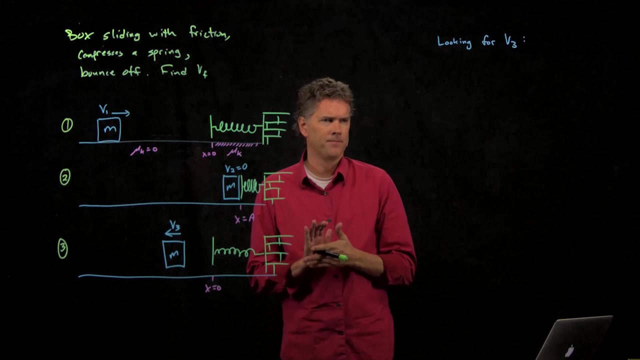 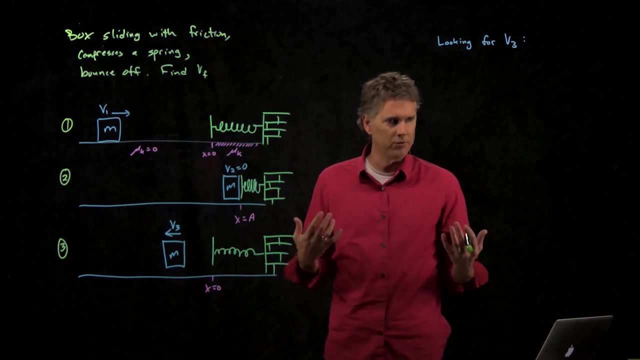 This is position 3.. So I need to think about some principles here to attack this. What is a good principle that we could use to attack this problem? Well, how about work? This whole chapter is called work. This is one of your chapter problems. 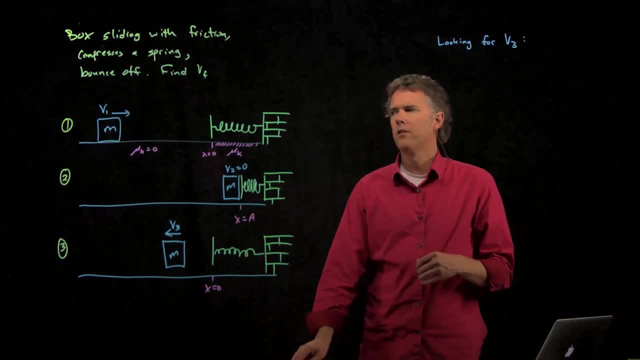 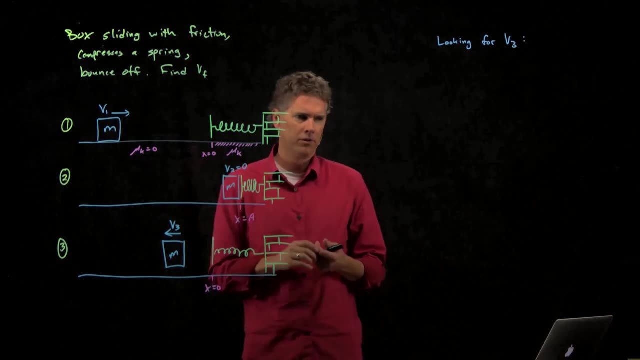 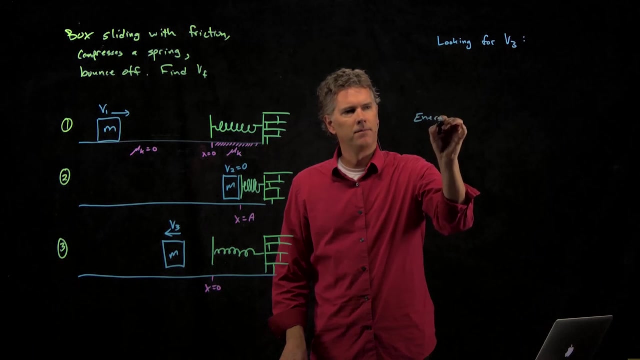 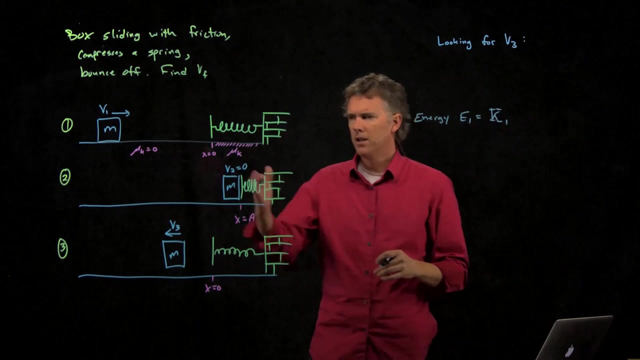 or at least it's very similar to one of your chapter problems. So let's think about this from the terms of work. First off, when we are heading into the spring, what sort of energy do we have? We have kinetic energy, And then it's going to compress the spring. 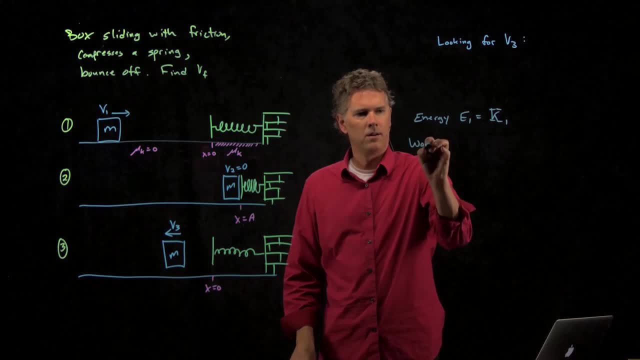 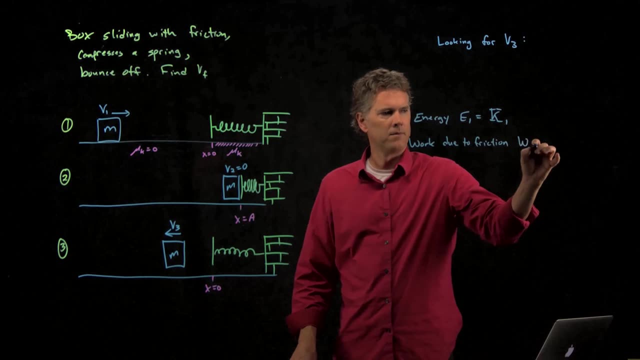 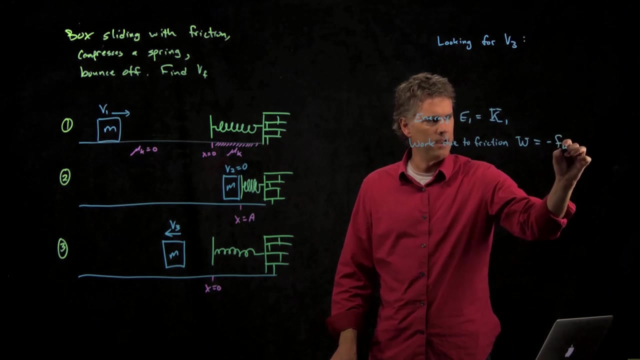 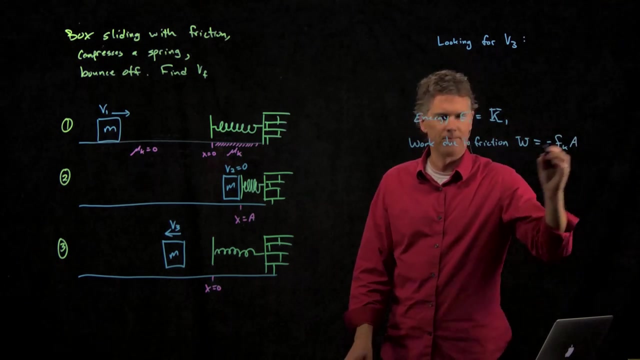 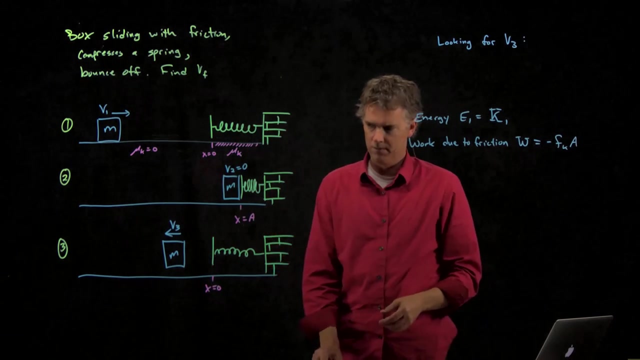 And so we're going to do work on it, because there is friction, And we know what that friction is: It's minus FK times the distance D that it goes, which in this case is the distance A, And then it's sitting here at this compressed position. 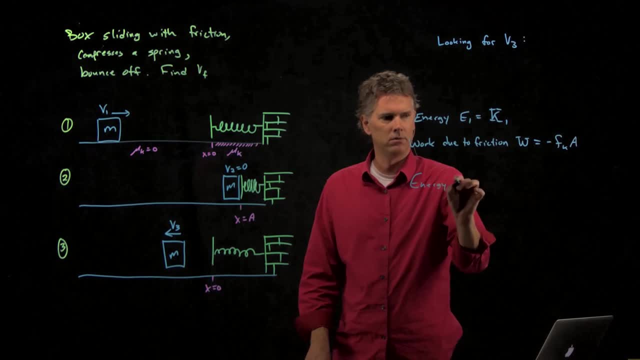 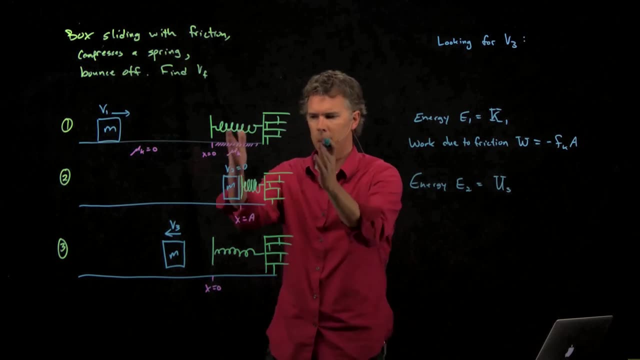 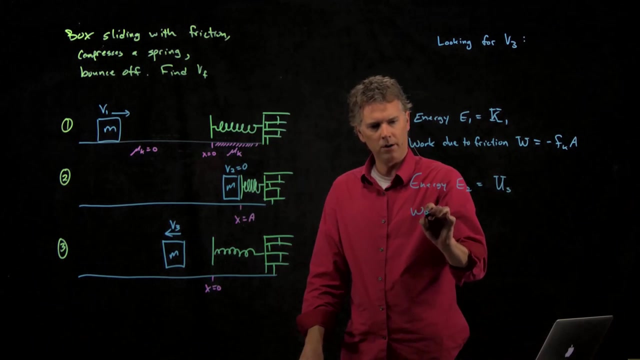 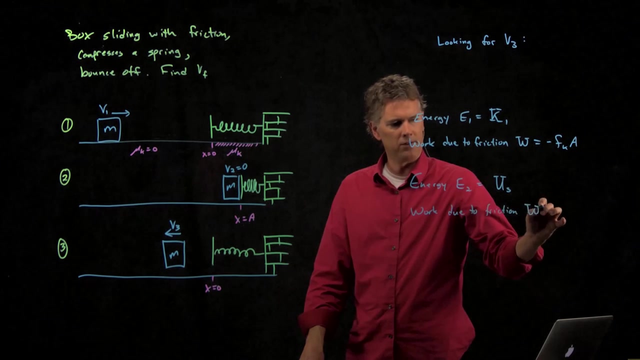 So the energy here at E2 is spring potential energy. Right, We have a compressed spring And then it's going to slide back out, And so in between these two we're going to do work due to friction, And again it's going to go across the same distance. A. 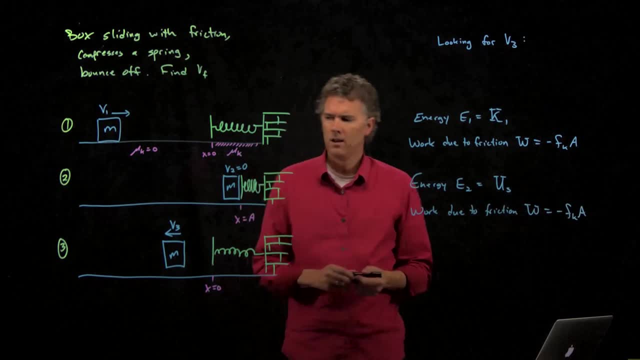 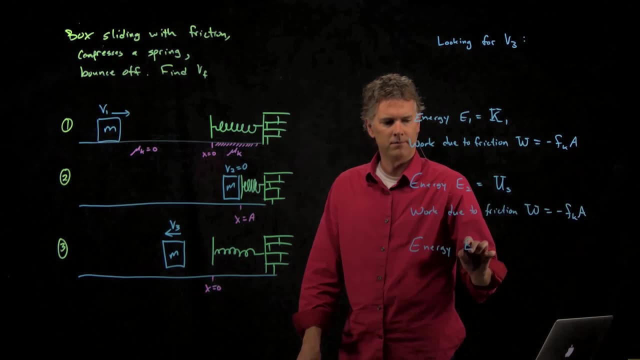 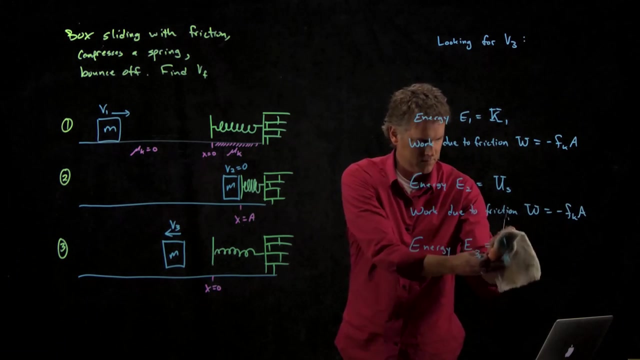 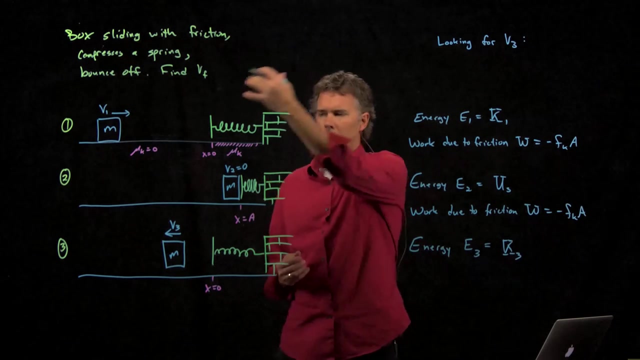 And so it's just minus FK times A, And then it's going to shoot off And so it's going to all go back to kinetic energy. So we come in with some kinetic energy, We're going to do some work on it. due to friction, 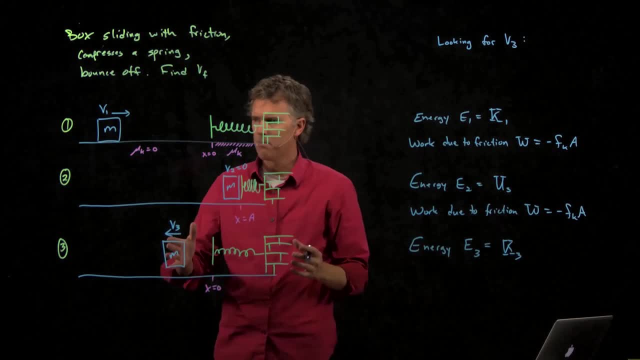 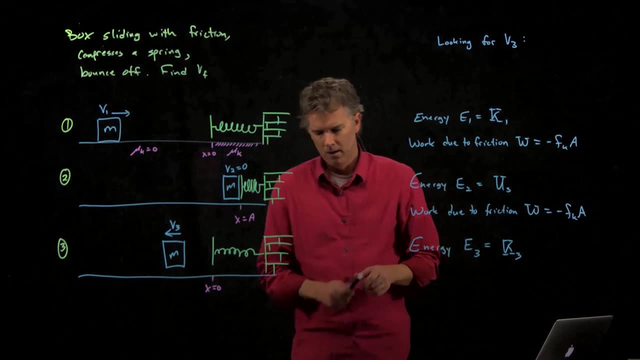 We're going to have some energy in the spring, It's going to return back out. Do some work on friction on the way back out, And then the box will slide along with kinetic energy. So one way to think about how to attack this is the following: 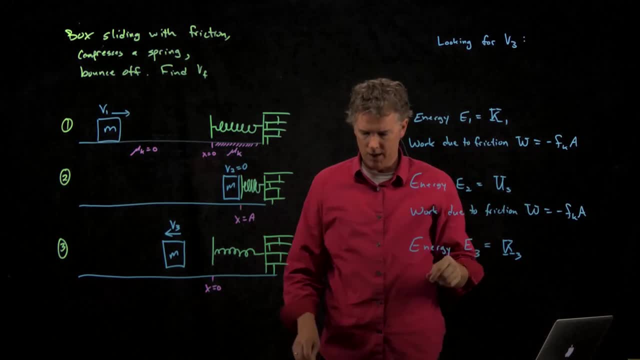 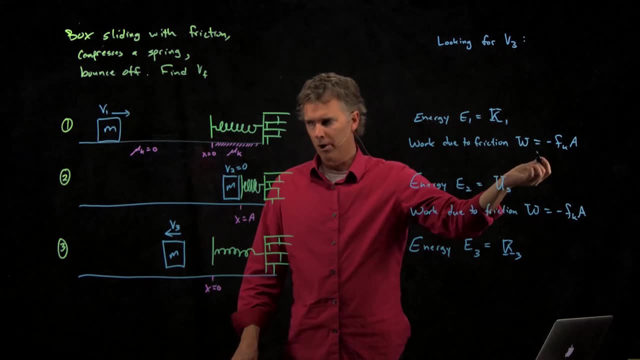 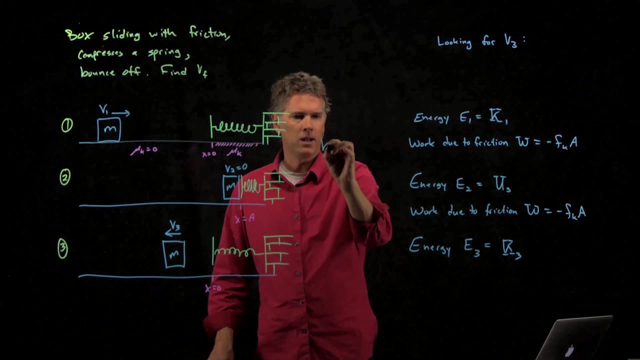 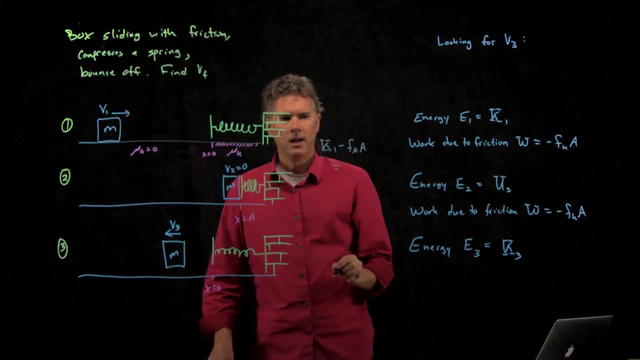 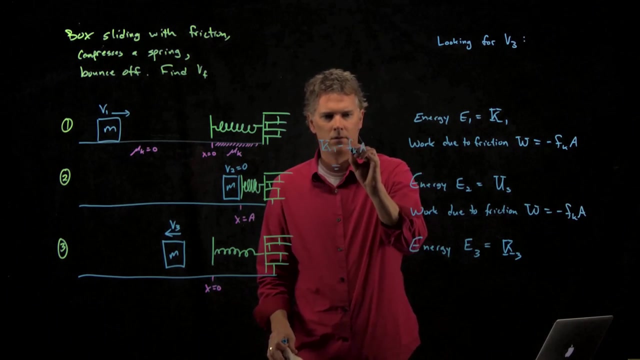 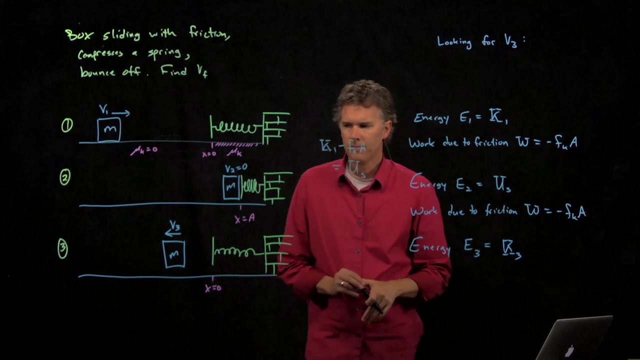 The energy in this first part is really just going to be whatever kinetic energy we have minus the work that we did. Okay, And so we could say that kinetic energy one minus FKA is going to be equal to whatever energy is stored in the spring. 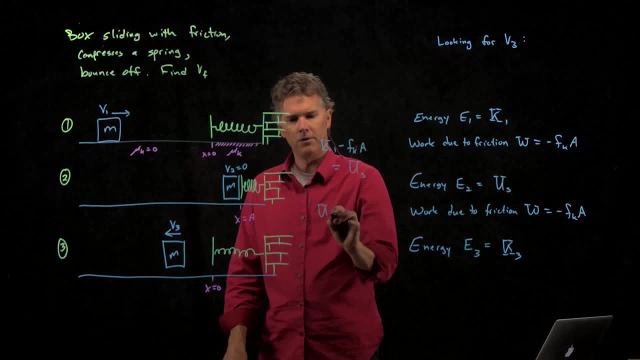 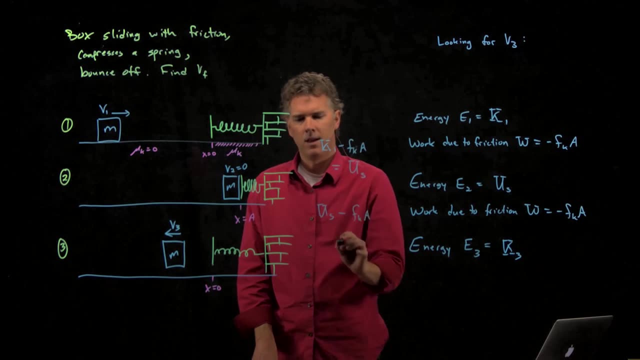 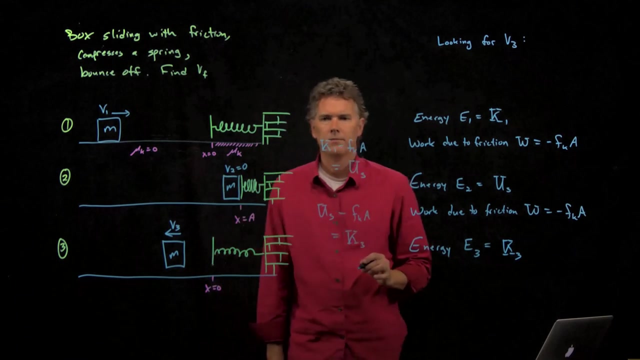 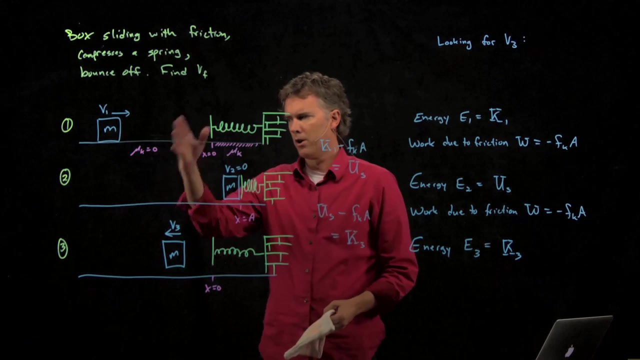 And now going from two to three, whatever energy is stored in the spring, we subtract FKA And that's got to be equal to the final kinetic energy, K3.. So how do we solve this problem, This idea of doing work and looking at energy and so forth. 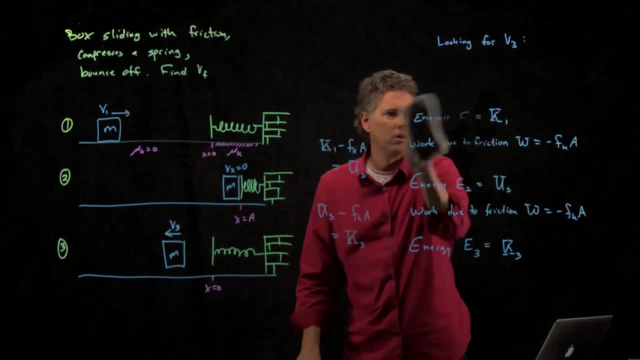 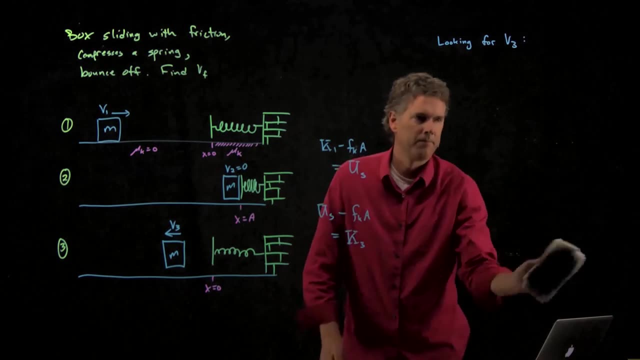 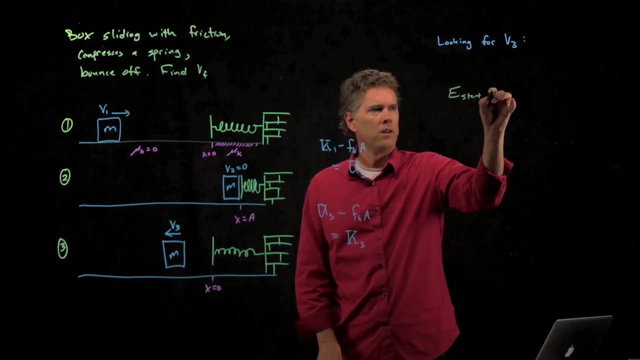 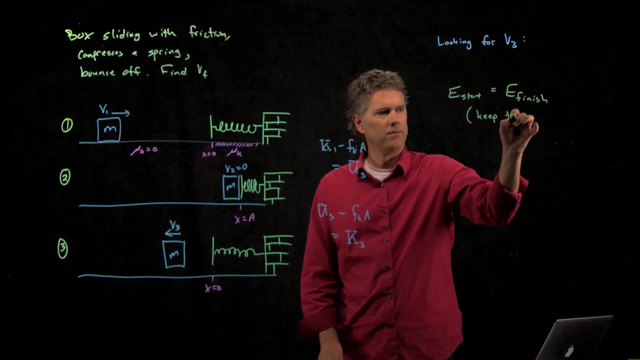 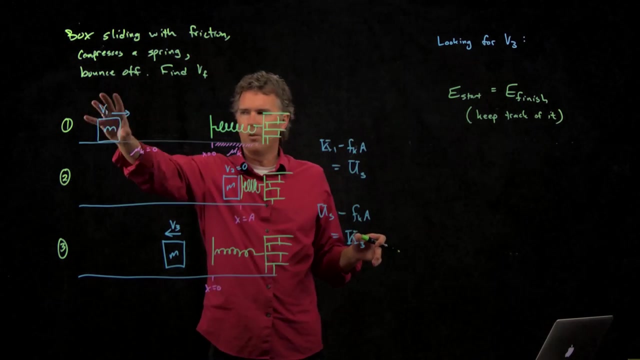 you can sort of be careful and illustrate it like this, or you could just say the following: The energy that I start with has to be equal to the energy that I finish with, as long as I keep track of it. And so let's look at the energy that we start with. 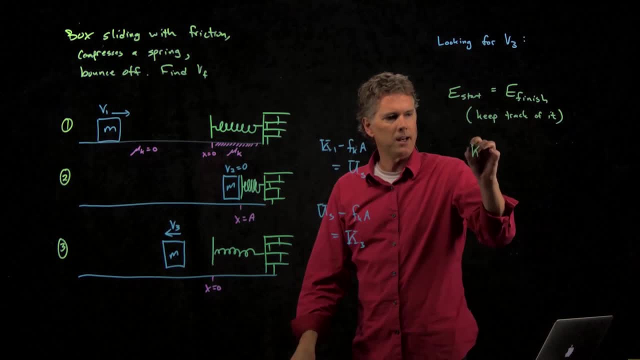 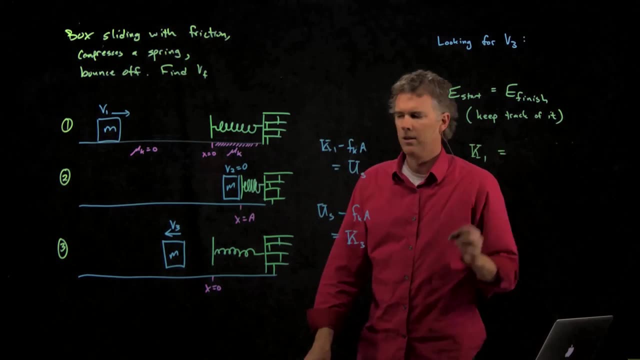 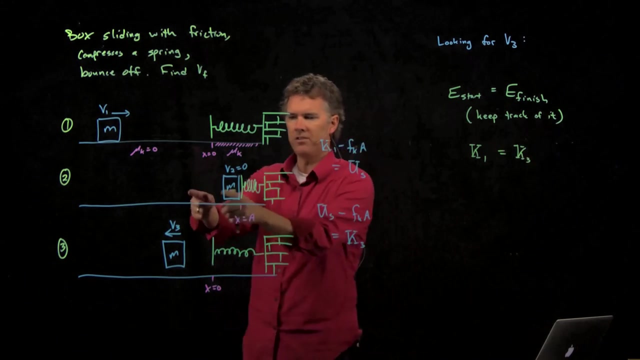 The energy that we start with is all kinetic energy. It is kinetic energy one, And now the energy that I finish with is going to be kinetic energy three. But we know that we slid across a frictional surface on the way in and on the way out. 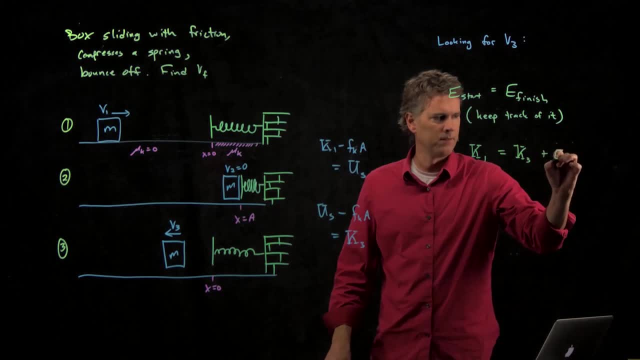 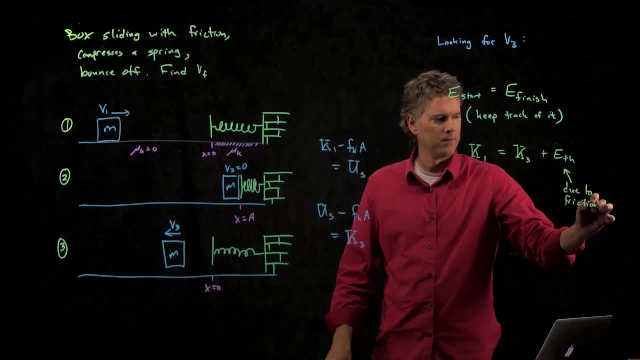 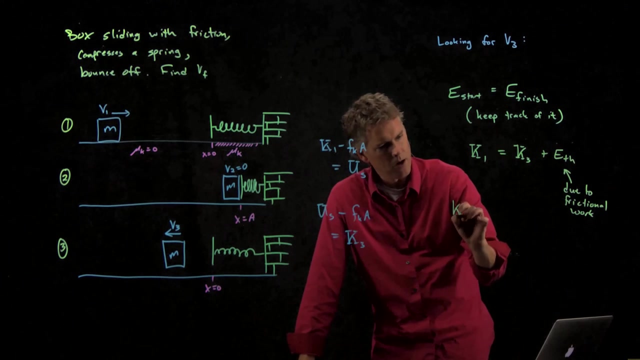 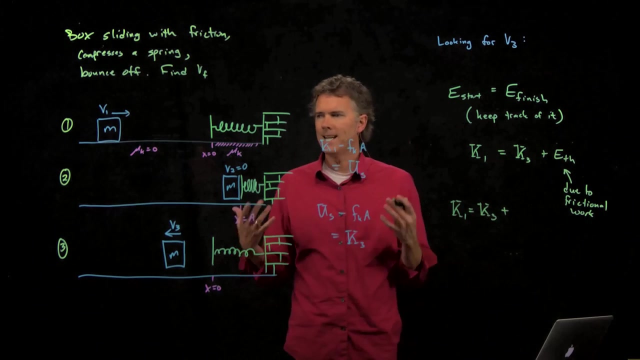 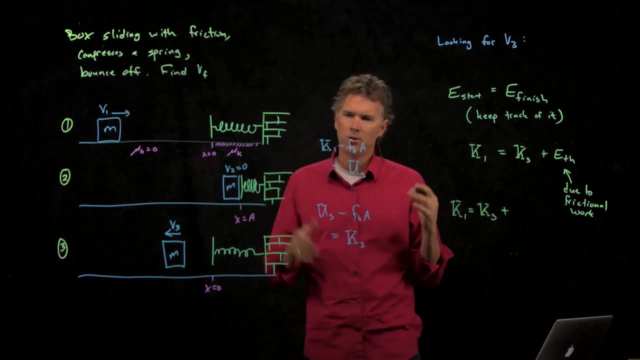 And so that is going to be thermal energy, And this is due to the frictional work. Okay, So K1 equals K3, plus whatever work I did due to friction. But thermal energy is a positive quantity, And so we need to worry about the magnitude of the thermal. 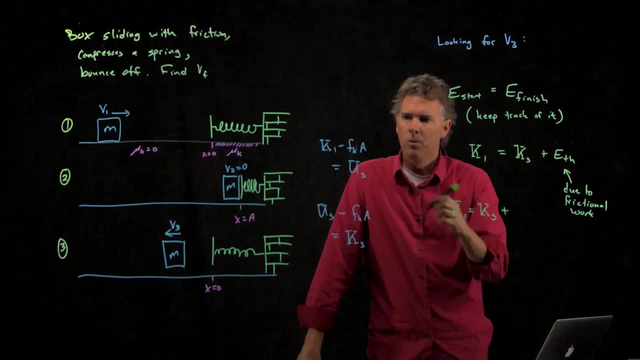 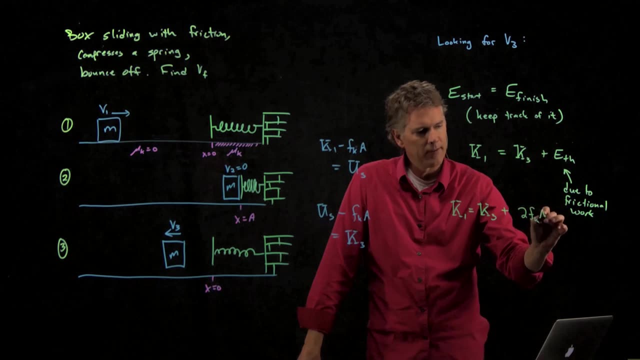 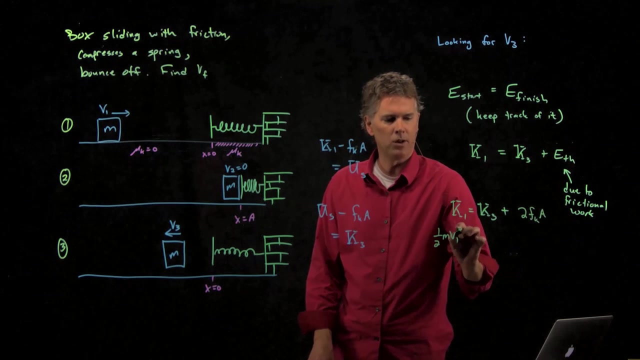 the magnitude of the frictional work. We know that we did FKA on the way in, FKA on the way out, And so this becomes two FKA, And now we see what we have. We have one-half m V1 squared.